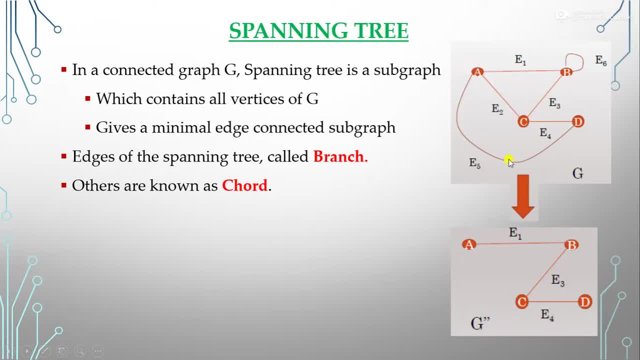 tree and the codes are like that: this ADE5 or E6 or E2.. So these are the code, right, which are removed to make the spanning tree. So this is called the code. So if we have this, example, G double dash is a spanning tree. So what are the branches of the spanning tree? So if we have this, 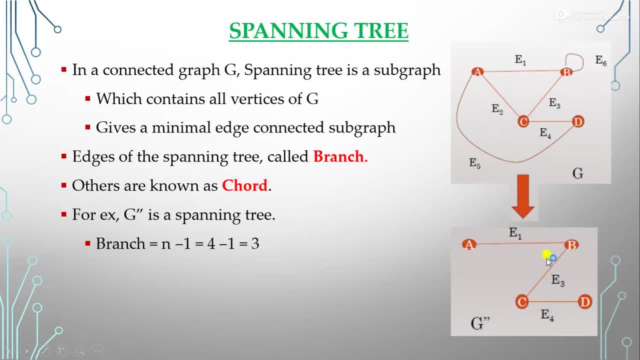 branch here. So branches because N vertices, four vertices are there, four minus one. three edges are three and we say that the edges of spanning trees are branch. So branches three here and code what is the code here? So you know that we remove how many edges to make the spanning trees E minus N plus. 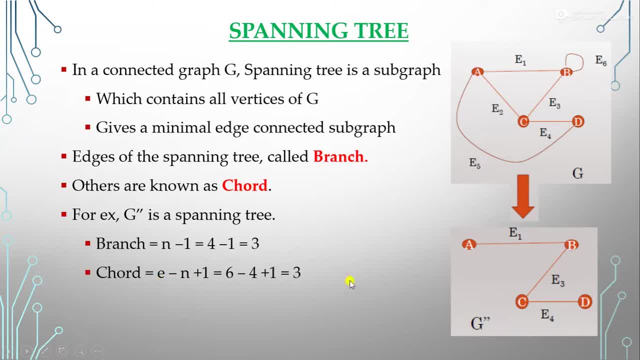 one I will. I told you earlier that. So E is the edges here, So edges here, edges E. it means that we remove how many edges to make the spanning trees, So that is six, and vertices are four and plus one, So it will give three. It means that the branch and code of the spanning tree is three, are three, and 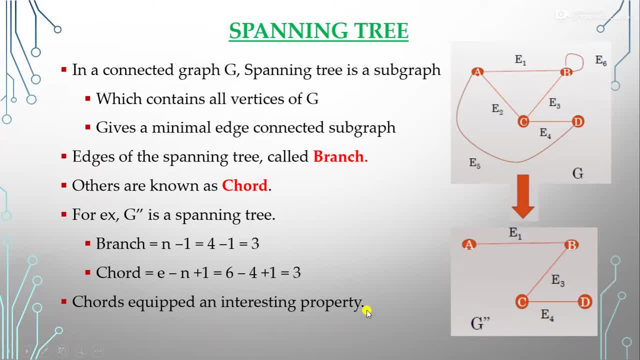 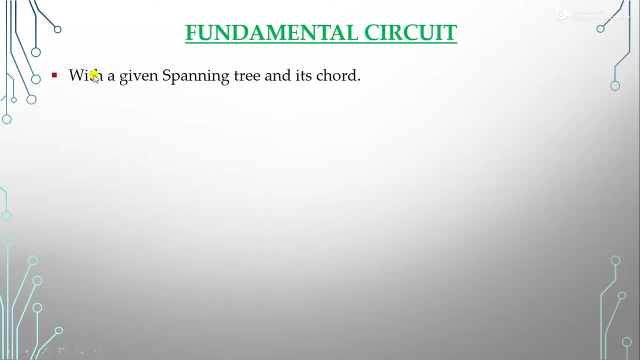 three. So here, code equipped an interesting property, means we use the code in our, the fundamental circuit. So what is the fundamental circuit? With a given spanning tree and its code, a circuit formed introducing every single code. So in a spanning tree, if we introduce a code, so a. 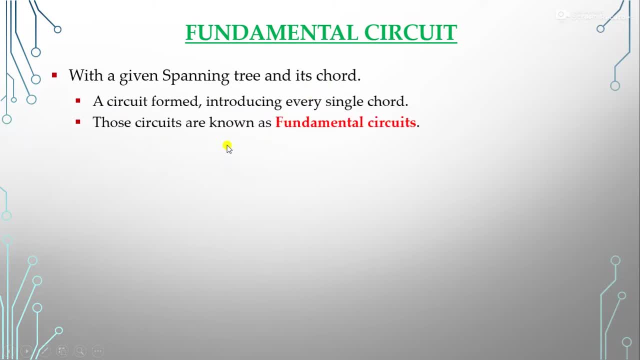 circuit can form, so that circuit is called the fundamental circuits. For example, suppose we have a spanning tree of the graph. this is our the graph, and the spanning tree of this graph is this one, suppose. okay, So here we have total, the five vertices are there and seven edges are there in. 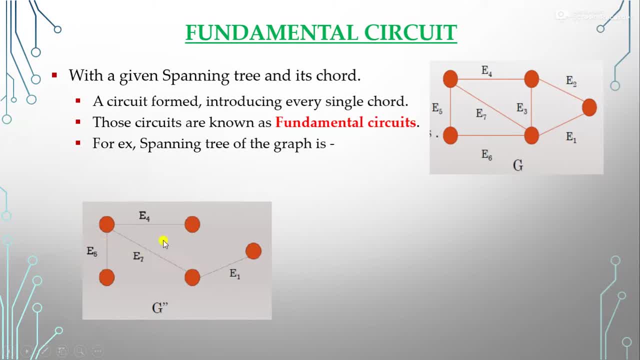 a given graph, If we say that this given graph, the spanning tree is this one Z double dash. So here in this graph, how many vertices are there? Five and edges total seven, and in this spanning tree graph we have, the vertices are five. So now, what is the branch and code here? Branch Branch is the edges. 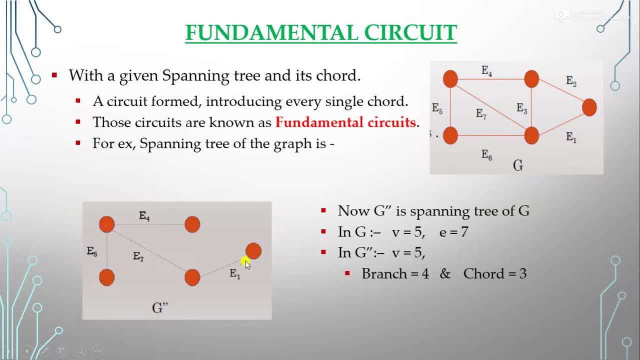 of the spanning tree and how many edges of the spanning tree? here Four, So branch is four. Now how many edges of the graph given, graph G. So that is three, right? or you can calculate by e minus n plus one. So from this you will get the three. and what are the codes here? The codes are which we 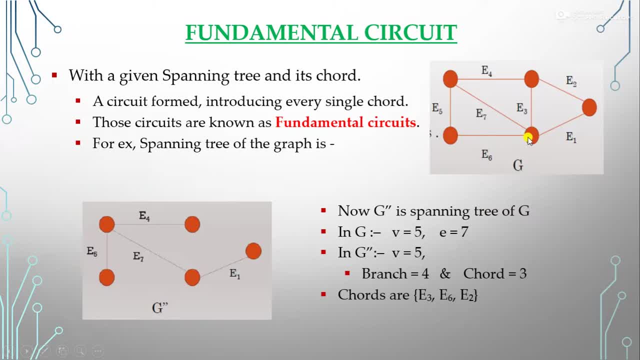 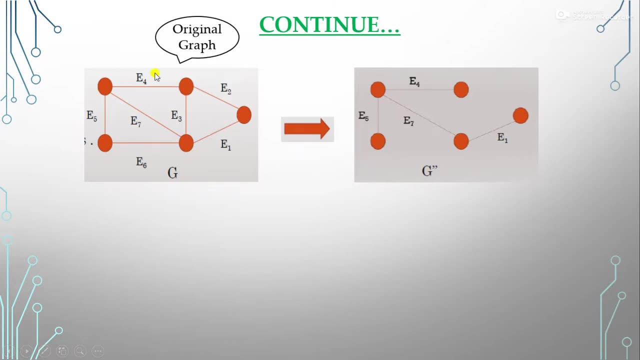 remove here that one: e3, e6, e3, e6 and e2.. So these are called the code of the graph: How to form the fundamental circuits. So this is our the original graph and this is is the spanning tree of this graph. So from the spanning tree, how can we form the fundamental circuits? 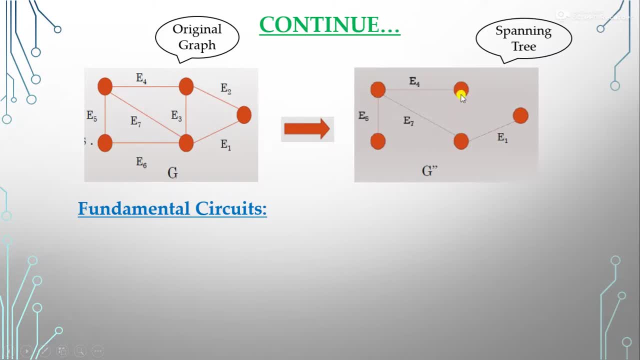 I told you that the fundamental circuits are that in which, if we add any code of the spanning tree which form a cycle, So that is the fundamental circuit. So first one is this: if we join these means we add this e2. So it become a cycle. So one fundamental circuit of this graph is this one. 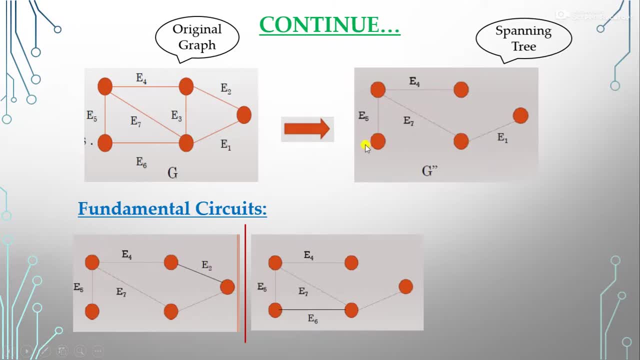 Another one. if we join this to this one means e6. So again it become a cycle. So one another fundamental circuit of this graph is this one and another one. if we join these two vertices means by e3, if we introduce here. So it become a cycle. So this is also. 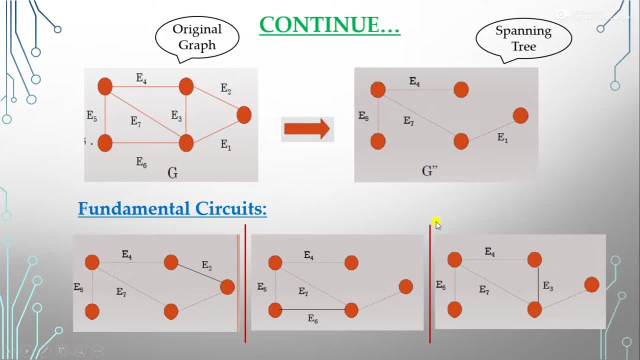 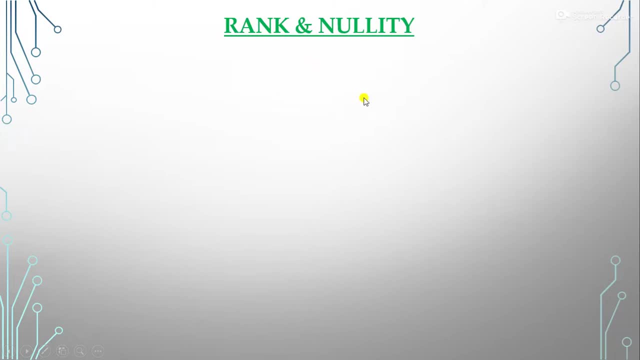 a fundamental circuit of this graph. Okay, clear it. what is the fundamental circuits? Now come to the rank and nullity. So what are the rank and nullity? First of all, we discuss about the rank. So what is the rank If in a graph G there are total, n vertices and k components? 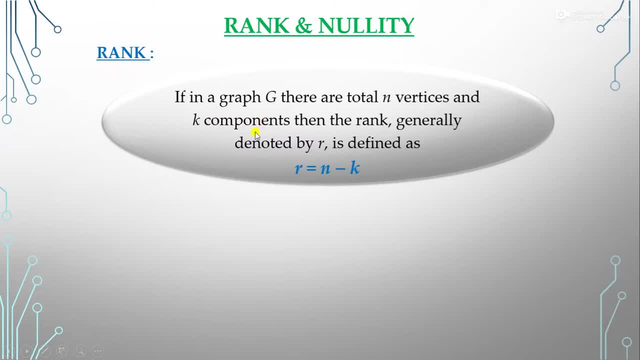 what is the components? Actually, I told you earlier that what are the components means, if we have a disconnected graph, So you have the two or three parts of that disconnected graph, So that is called the components. Then the rank generally denoted by r, small r, and it is defined as n minus k, n is the total number of. 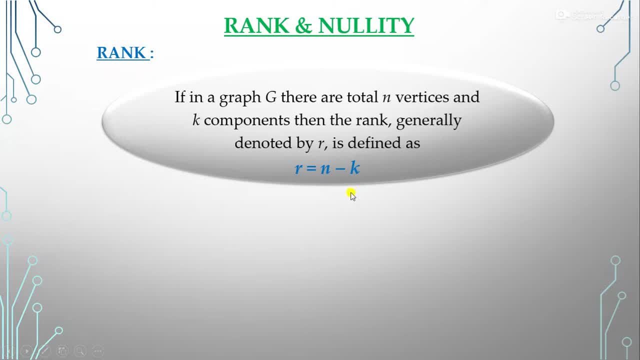 vertices and k are the components of the graph. Here we talk about the disconnected graph. Then it is n minus k, Now nullity. What is the nullity? If in a graph G there are total n vertices, k components and E ages, then the nullity. 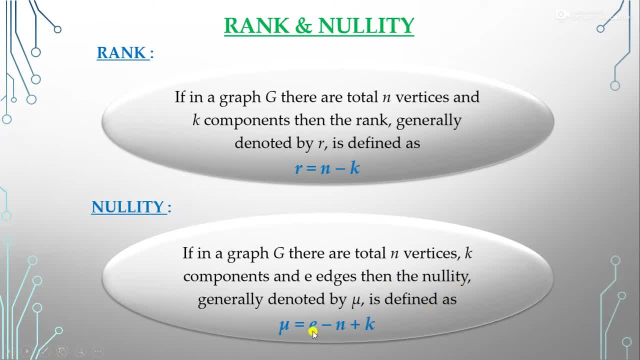 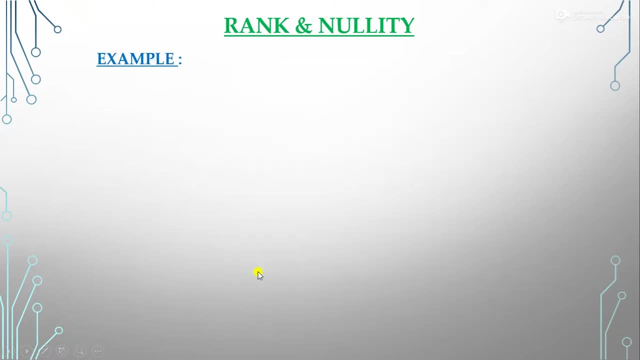 it is denoted by mu and is defined as E minus n plus k. E are the edges of the graph, n are the vertices and k are the components. So this is all for the disconnected graph. So now let's take an example here. if we have this disconnected graph G and here this is: 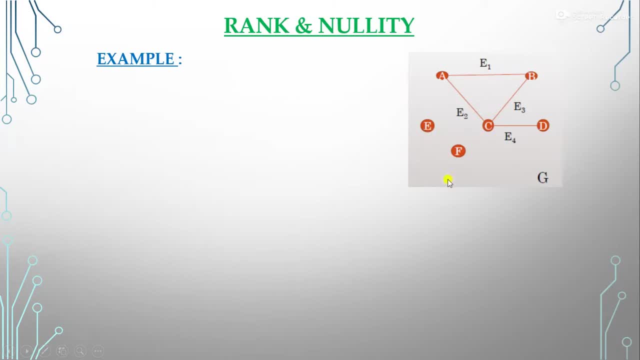 disconnected because these vertices are disconnected with these vertices, not joined with any edges, with all vertices right now in this graph g, what is the rank? i told you that rank is n minus k. n is here. four vertices means we have to take, we have to consider that vertices which 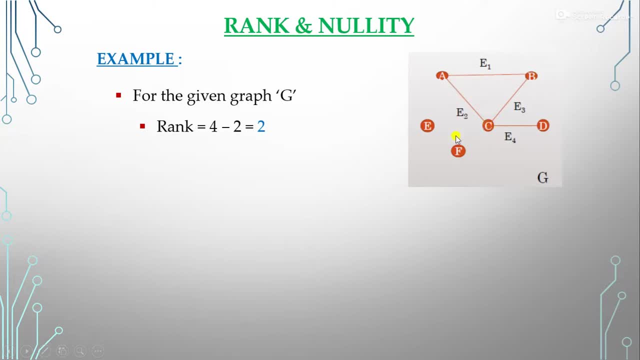 are connected, right, so four minus two k. here is two y components, two components. this graph is divided into the two components. one is this one and one is this one, right, so our rank is two. now nullity. nullity is e, e is the edges. four edges are there minus n and the four vertices. 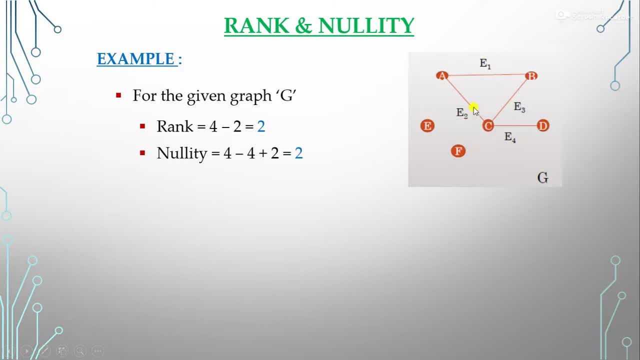 are there plus k. k is the two here, right? two components of this here. so this is four minus four plus two it become two. so the rank and nullity of this graph is two and two. now one point here. this is for disconnected graph. suppose we have the connected graph, so in the connected graph 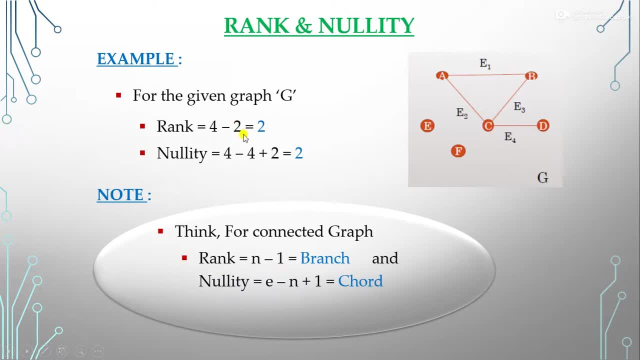 rank is n minus one, because if we put here k is equal to one, so we get the rank for the connected graph and this is our, the branch also, i told you earlier. and nullity is e minus n plus one become and it is equal to code right. hardly i solved it, so now we can. 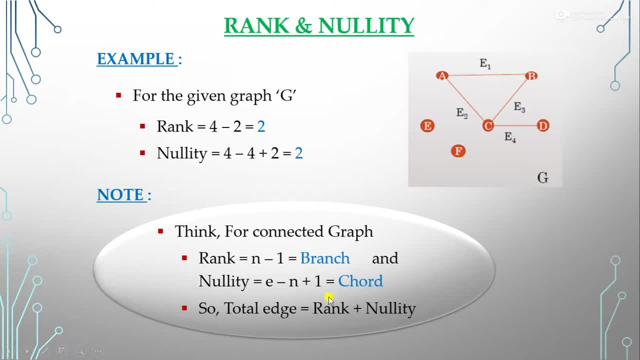 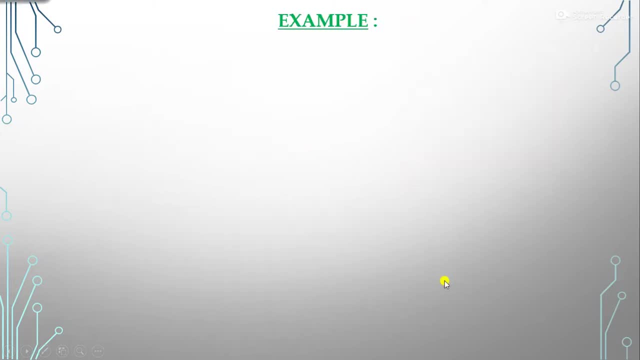 say that the total edges is equal to rank plus nullity. clear it. this is for the connected graph only. so now let's take one example. actually, this is the example for the trees, and this is a very important example here. if say that a tree has two vertices of degree 2, one vertex of degree 3 and 3. vertex of degree 2. and because thisardanal Speyer of trie has two vertices of degree two, one vertex of degree three and three, vertex of degree three, that takes the wrong axis, which is n minus k günü, and that is n. coverage from the vector Sa is equal to. 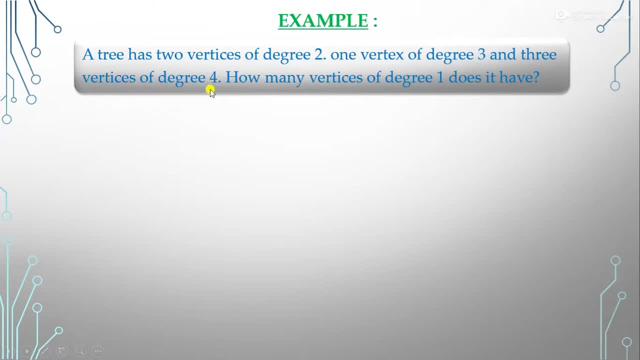 x más n equal to gray. the next right example: we have signalal Art of University in the and 3 vertices of degree 4, then how many vertices of degree 1 does it have? So now you have to calculate the vertices which has the degree is 1.. So now let's do it First. 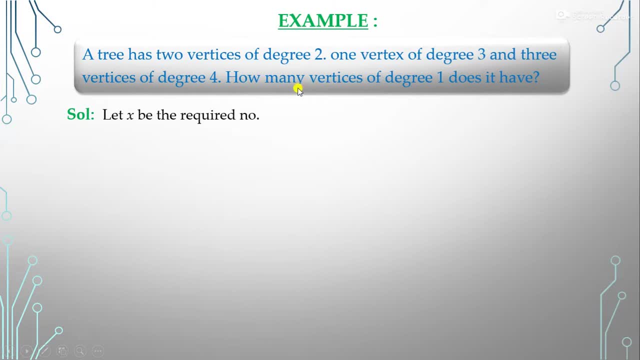 we consider that, suppose, which we want to find. we consider that is x, right, So now, how many total number of vertices here? 2, 1, 3 and 1.. So 2 plus 1 plus 3, and here, when we use the vertices, 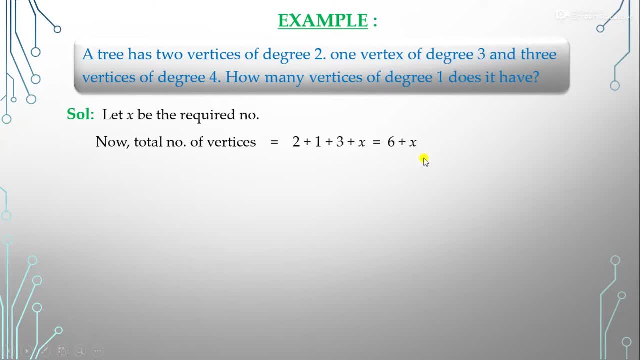 x. So total, we have the 6 plus x vertices are here. Now the number of edges: how many edges are here? We say that because a vertices is 6 plus x, so edges are in the tree. you know that. 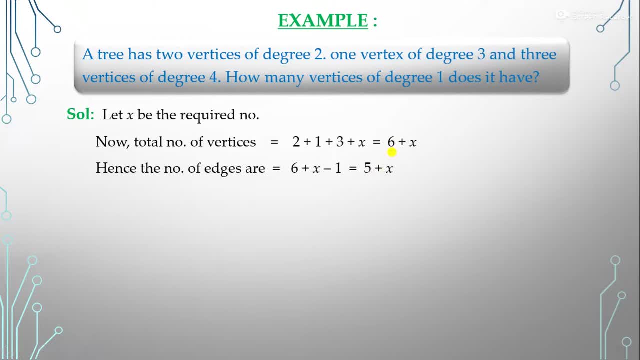 if we have the n vertices, then edges are n minus 1. so if we have the vertices, 6 plus x, so edges are 6 plus x minus 1, so it becomes 5 plus x. so in this tree total number of edges are 5 plus x. and why? because 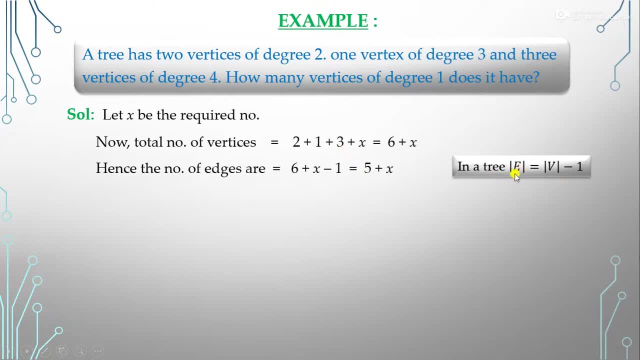 we know that the in the tree the number of edges. this is equal to the number of vertices minus 1. now total degree of the tree. so what is the degree here? 2 total vertices. 2 vertices have degree 2. it means that total degree is 2 multiply 2. 1 vertex has degree 3 plus 1 multiply 3- 3.